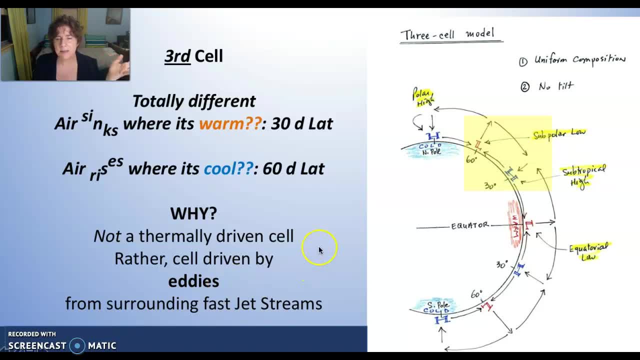 Look at this cell in the middle. It's completely different. The rising air is up in the cold 60s. The sinking air is up in the relatively warmer 30s. That doesn't make sense. Rising air should be warm, Sinking air should be cold. Why is there even a cell here? It's not thermally driven. 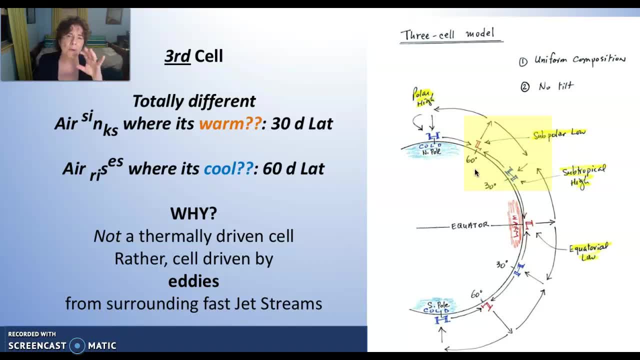 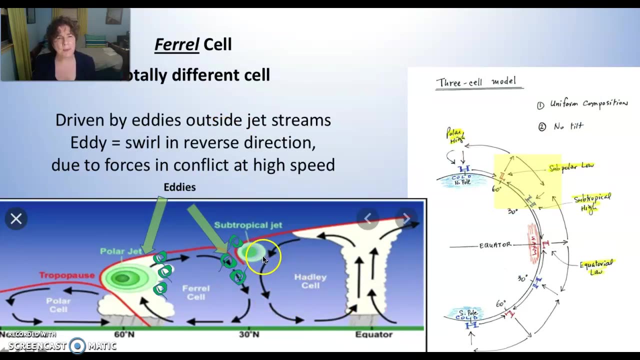 It's actually driven. It's actually driven by eddies from the fast jet streams that border both sides of the ferrule cell. Let's look into that a bit. This schematic will really help you out. When we have the Hadley cell, we know as it sinks it develops into a subtropical jet. 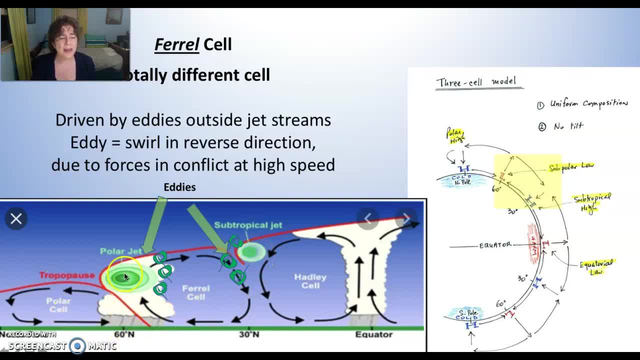 When we look at the polar cell, we know that as this air rises due to the convergent warm and cold air in the 60s, we also have a very strong polar jet. due to that gradient, These jets can be so fast that they set in play eddies, And eddies are swirls of air. 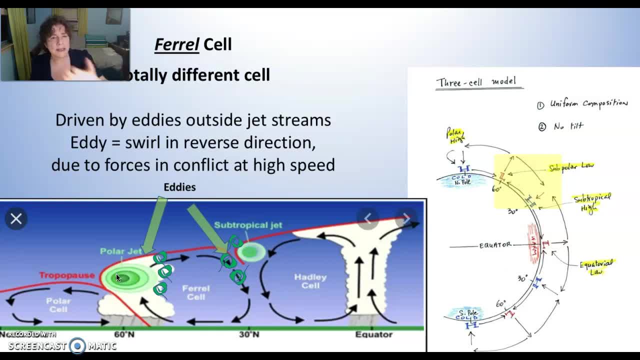 that produce turbulence because they opposite. they work in the opposite direction of the regular flow. In many cases, when you have forces at high speed, you'll find eddies around it And the eddies can do quite a job. We'll look into that a little bit more soon. Let's look into it a bit now. 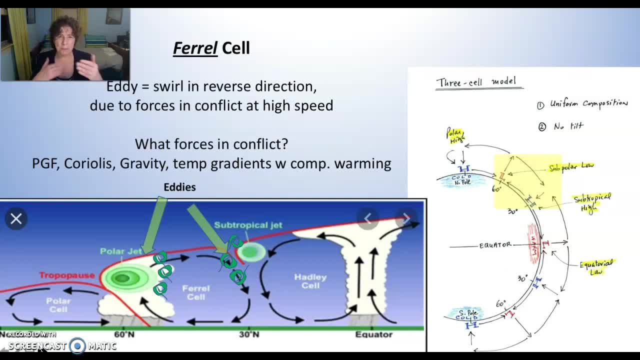 What forces are we talking about that might be in conflict at these high speeds, in these, in this polar jet? Let's talk about the forces that we know. We know that there's a pressure gradient force going from south to north, going from warm air to cold air. 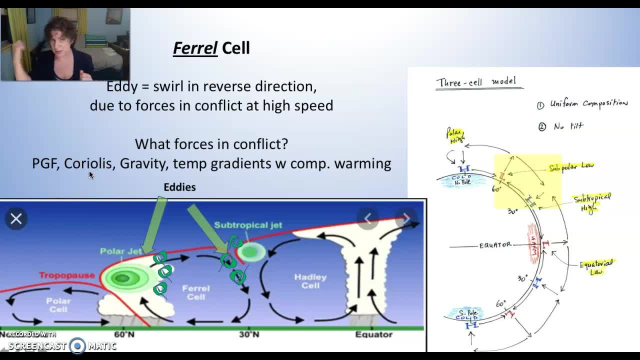 We know that there's a Coriolis force deflecting to the right. The Coriolis is faster the greater speed you have and the greater differential between the two weather conditions. We know that there's gravity as a force at play with this jet. 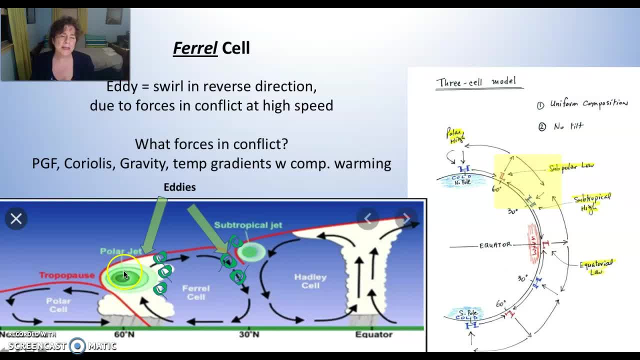 Gravity is everywhere and we know that there are some areas in here which will be dealing with compressional warming as this air starts to sink. Not as important, But it's there a bit. So the three big ones are the pressure gradient force, the Coriolis force, the gravity force At 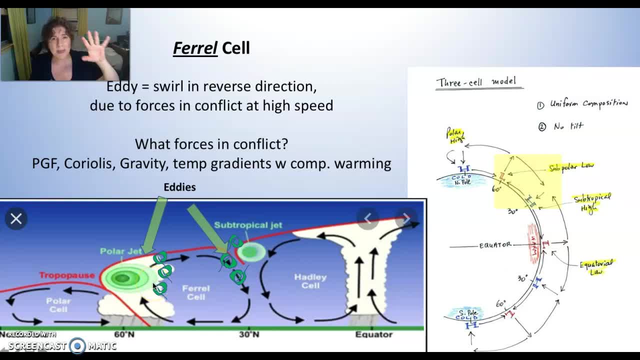 miles an hour. some things can go haywire, some things can go in reserve course. i drew some eddies out here for you. this is what causes turbulence at 30 000 feet, this eddy motion that we're talking about, this circular motion in the opposite direction, something that we can look at. 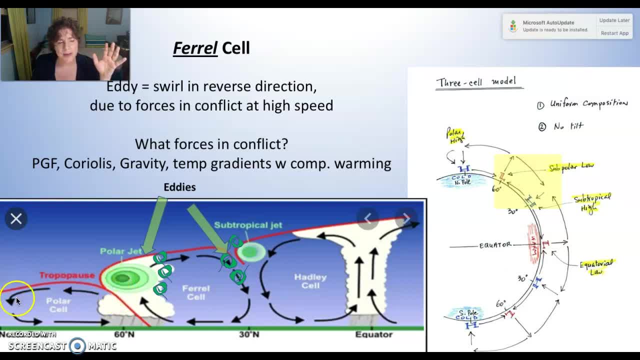 when we look at the direction of the polar cell. the direction of the polar cell is in a counterclockwise motion and the polar jet will go in a counterclockwise motion, but it'll go on a westerly course. right, it'll go on a westerly course. the counterclockwise motion, the eddies. 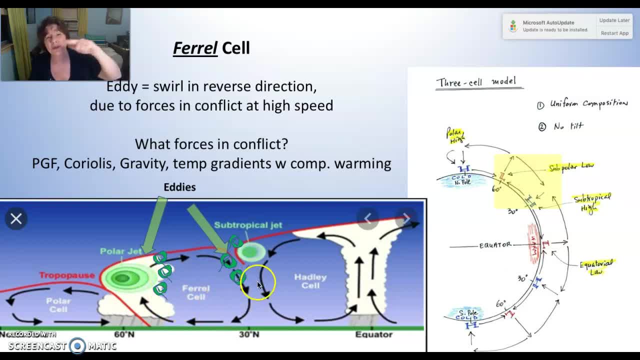 on the other hand, will go in a clockwise motion because they'll go in the opposite direction. same thing here from the hadley cell. we have a really strong hadley cell. here we have a weaker subtropical jet. that weaker subtropical jet is an. a weaker subtropical jet is an. 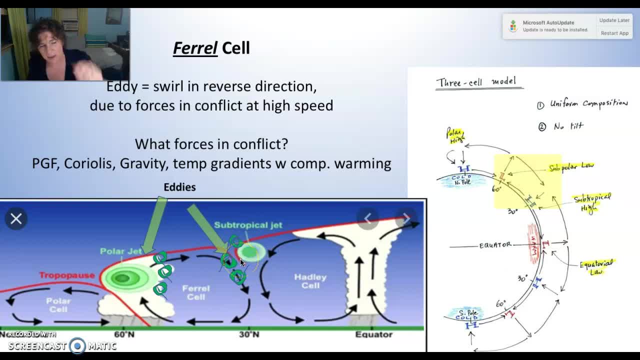 a weaker subtropical jet is an a clockwise direction, but it's also heading a clockwise direction, but it's also heading a clockwise direction, but it's also heading on a westerly course. these will these eddies on a westerly course. these will these eddies. 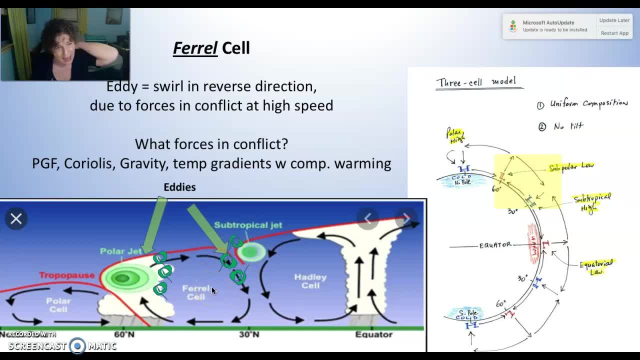 on a westerly course. these will, these eddies that come off of this fast jet, not as fast. that come off of this fast jet, not as fast. that come off of this fast jet, not as fast or as powerful as the polar jet. these will. 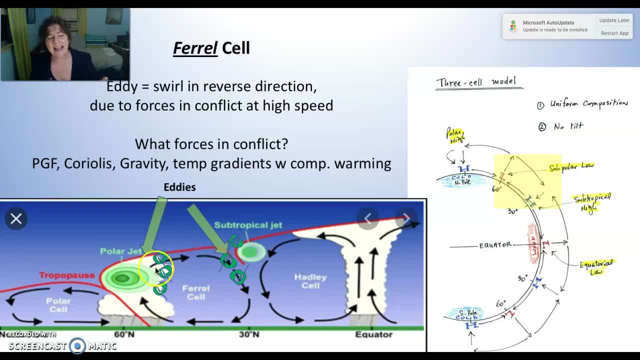 or as powerful as the polar jet, these will, or as powerful as the polar jet, these will also support a clockwise motion that has also support a clockwise motion that has also support a clockwise motion that has no basis in the thermally driven cell. no basis in the thermally driven cell. 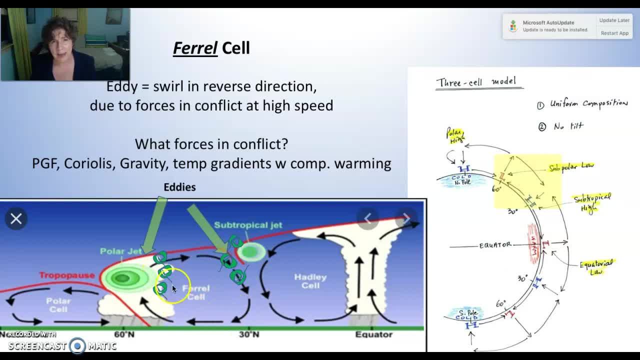 no basis in the thermally driven cell, strictly driven by eddies, and how strictly driven by eddies and how strictly driven by eddies and how powerful they can be from the upper powerful. they can be from the upper powerful, they can be from the upper atmosphere and the jet streams. 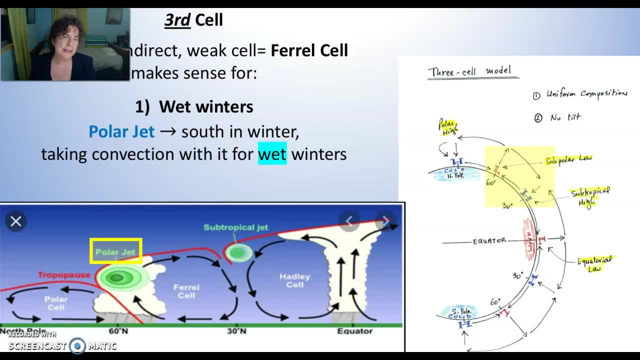 when we talk about, when we talk about, when we talk about the third cell, it does a lot to explain the third cell. it does a lot to explain the third cell. it does a lot to explain some of the wet winters that we know, some of the wet winters that we know. 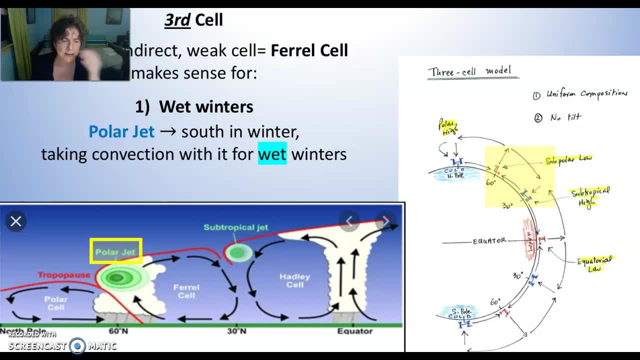 some of the wet winters that we know about in our area around the 40s, about in our area around the 40s, about in our area around the 40s, um and in particular up north of us in um and in particular up north of us in. 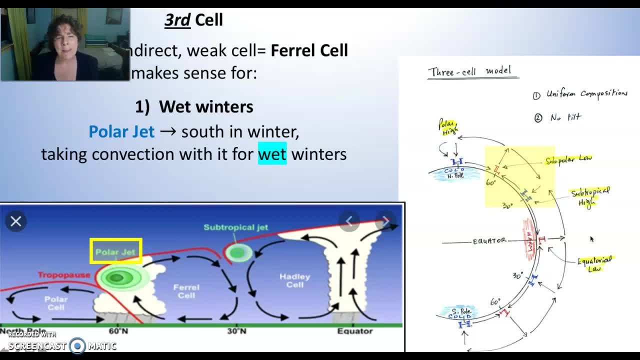 um, and in particular up north of us, in vermont and so forth, getting up toward vermont and so forth, getting up toward vermont and so forth, getting up toward the 60s, the 60s, the 60s. it explains, it explains, it explains wet winters for us. 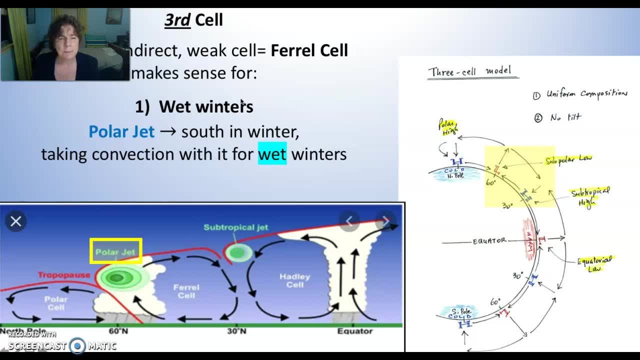 wet winters for us, wet winters for us. so this model seems to explain wet, so this model seems to explain wet, so this model seems to explain wet winters, winters, winters. because in the winter time, because in the winter time, because in the winter time the polar cell will move south with all. 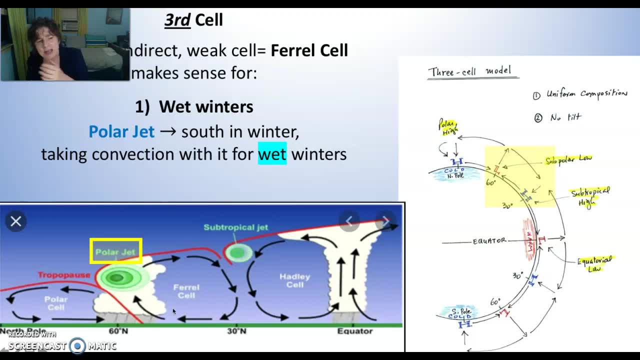 the polar cell will move south with all the polar cell will move south with all the cold air, the cold air, the cold air from the north pole, from the north pole, from the north pole. so, in moving south, it's going to move. so, in moving south, it's going to move. 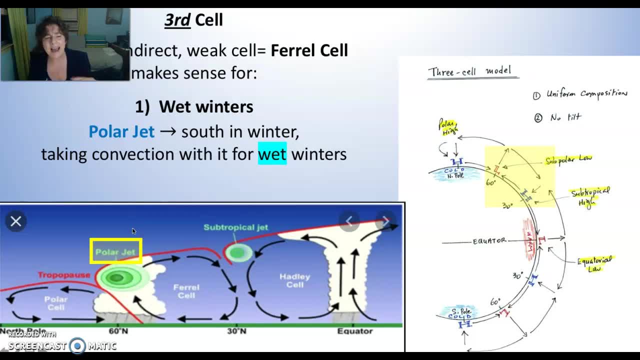 so, in moving south, it's going to move this convected area, this rising air, this convected area, this rising air, this convected area, this rising air rising slow, rising slow, rising slow um clouds and snow, um clouds and snow, um clouds and snow. surface low, it's going to move it down. 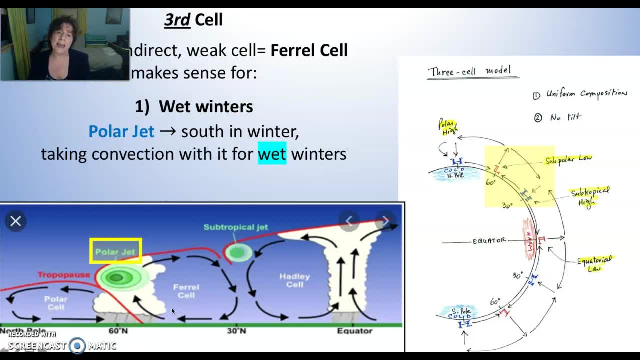 surface low. it's going to move it down surface low. it's going to move it down south of 60, south of 60, south of 60 and it will probably be in the area and it will probably be in the area and it will probably be in the area around vermont, around new york. that. 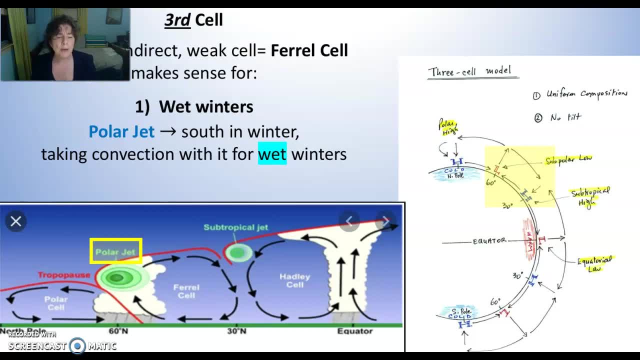 around vermont, around new york, that around vermont around new york, that makes sense for the wet winters, that we makes sense for the wet winters, that we makes sense for the wet winters, that we notice this model, notice this model. notice this model may really, um, may really help us out. 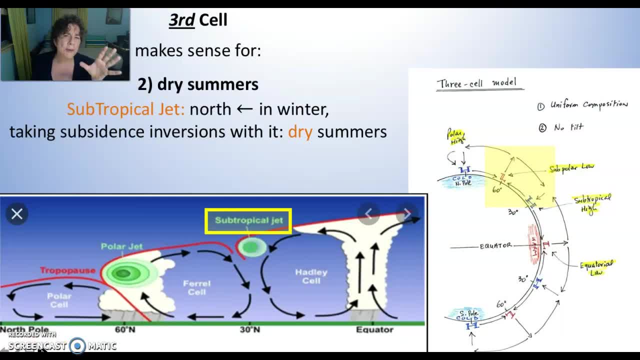 may really, um may really help us out. may really, um may really help us out quite a bit, quite a bit, quite a bit. and the third cell also explains the dry. and the third cell also explains the dry. and the third cell also explains the dry summers that we generally have around. 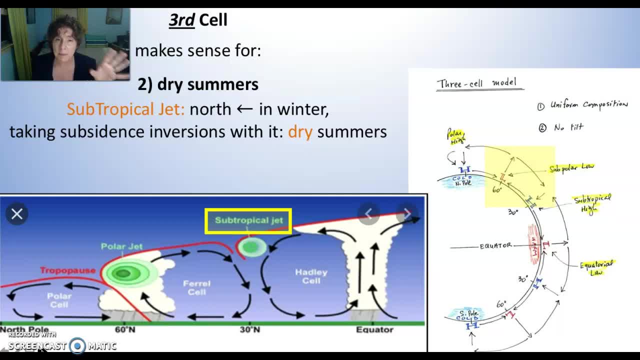 summers that we generally have around, summers that we generally have around our area, our area, our area, and particularly the dry summers that, and particularly the dry summers that, and particularly the dry summers that you notice up in vermont, you notice up in vermont, you notice up in vermont, um. so in the summer, the warm, 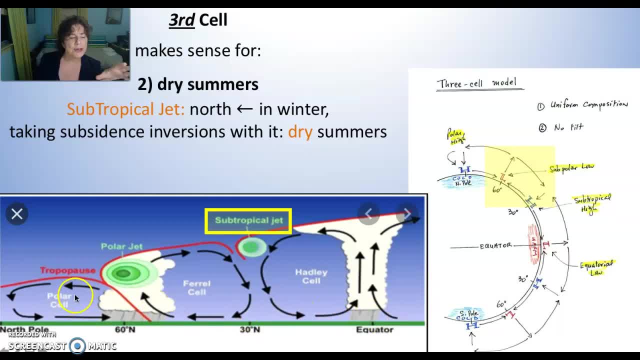 um so in the summer, the warm? um so in the summer, the warm air from the equator has more of a push. air from the equator has more of a push. air from the equator has more of a push and pushes the polar cell further north. 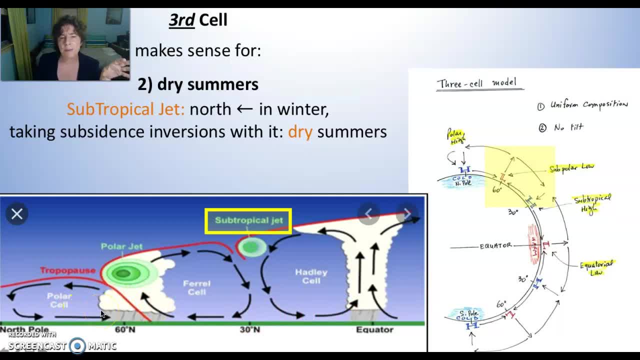 and pushes the polar cell further north, and pushes the polar cell further north. and in pushing the for and in pushing the for and in pushing the for the um the uh polar cell further north, the um the uh polar cell further north, the um the uh polar cell further north, we push. 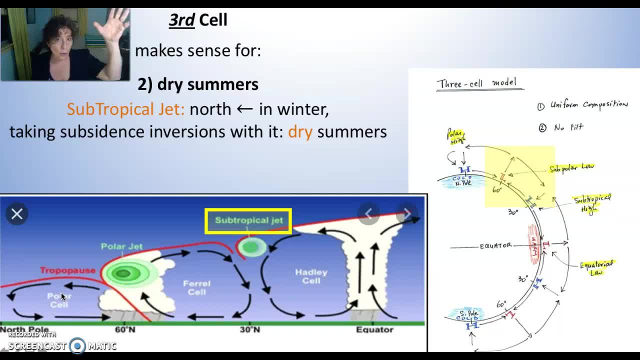 we push, we push the convection and the rising slow clouds, the convection and the rising slow clouds, the convection and the rising slow clouds, and snow, and snow, and snow up closer to the 60s and we give up closer to the 60s and we give. 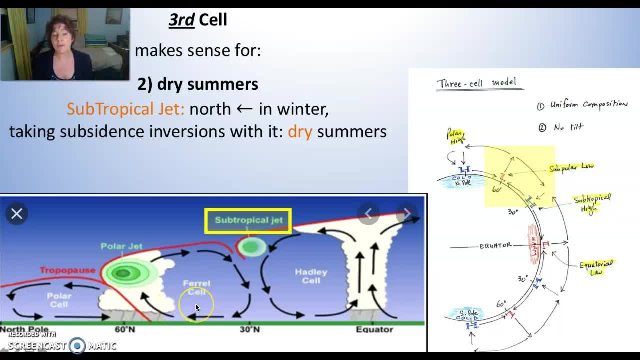 up closer to the 60s and we give ourselves ourselves ourselves, the dry area of the middle feral cell, the dry area of the middle feral cell, the dry area of the middle feral cell. so it can explain our dry summers. so it can explain our dry summers. 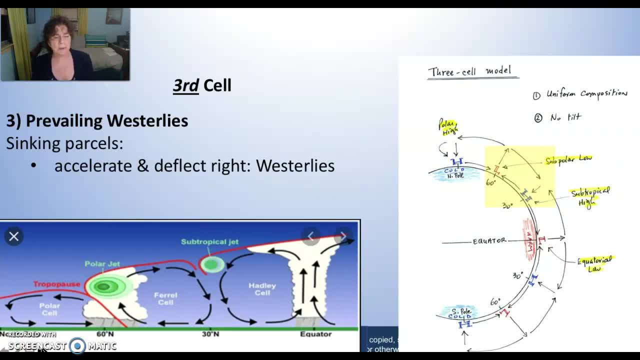 so it can explain our dry summers. and in addition, um, it'll definitely and in addition, um, it'll definitely and in addition, um it'll definitely explain the prevailing westerlies of the. explain the prevailing westerlies of the. explain the prevailing westerlies of the jet stream. 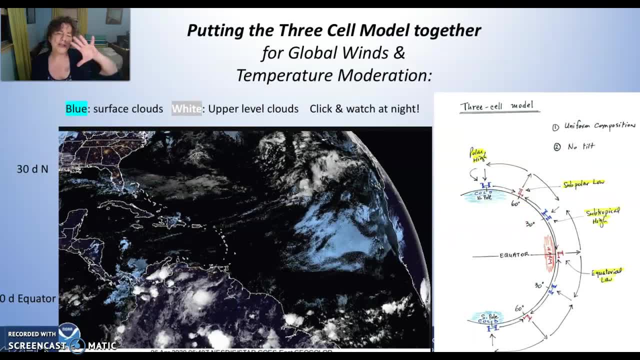 jet stream. jet stream, that's a given, and that's a given, and that's a given. and i wanted you to put all three of these. i wanted you to put all three of these. i wanted you to put all three of these cell models together. cell models together. 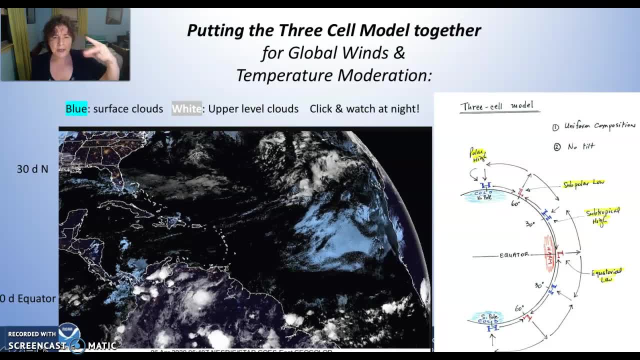 cell models together: the hadley cell, the polar cell, the feral, the hadley cell, the polar cell, the feral, the hadley cell, the polar cell, the feral cell, cell, cell, to understand, to understand, to understand that they move all the air within a, that they move all the air within a. 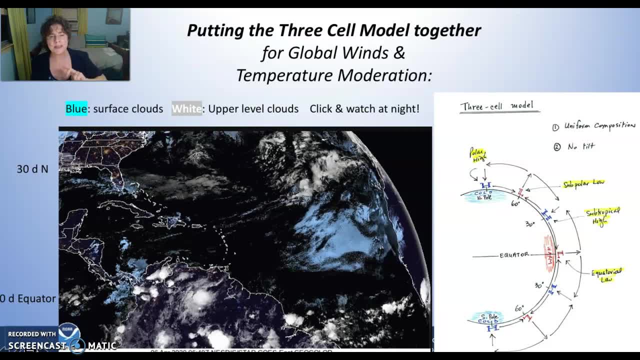 that they move all the air within a hemisphere, hemisphere, hemisphere. all of these working together, move this. all of these working together, move this. all of these working together, move this. the air and hemisphere. this is actually the air and hemisphere. this is actually the air and hemisphere. this is actually the ghost satellite at night. 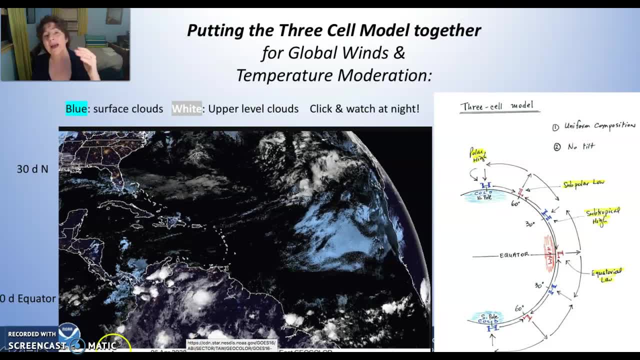 the ghost satellite at night, the ghost satellite at night which can pick up ir, which can pick up ir, which can pick up ir and will pick up even ir from low clouds and will pick up even ir from low clouds and will pick up even ir from low clouds and ir from high clouds. it's a beautiful. 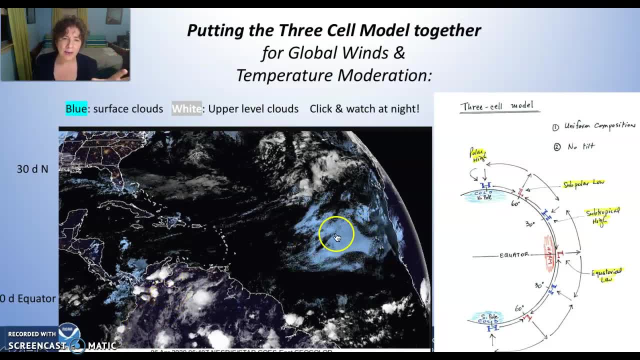 and ir from high clouds, it's a beautiful and ir from high clouds, it's a beautiful exhibit at night. and not only that, but exhibit at night. and not only that, but exhibit at night. and not only that, but the low clouds which probably are, the low clouds which probably are. 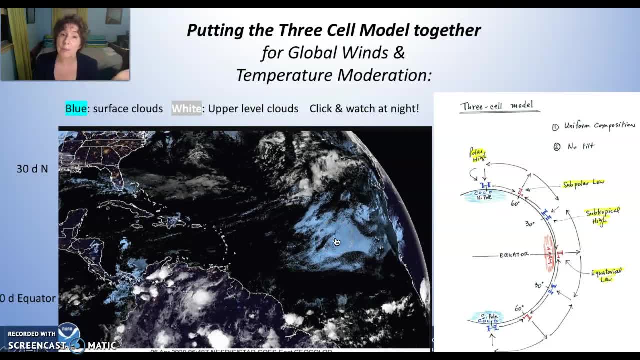 the low clouds which probably are associated with stratus clouds and associated with stratus clouds and associated with stratus clouds, and precipitation: precipitation: precipitation are blue and the high clouds which are are blue and the high clouds which are are blue and the high clouds which are probably. 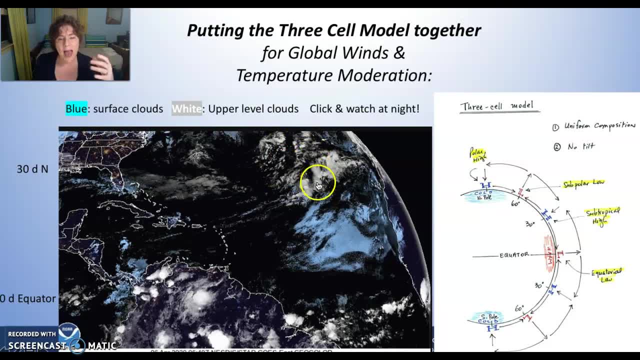 probably, probably, associated with ice and cirrus clouds. associated with ice and cirrus clouds, associated with ice and cirrus clouds are white, are white, are white, and what you see here is you see surface and what you see here is you see surface and what you see here is you see surface movements. 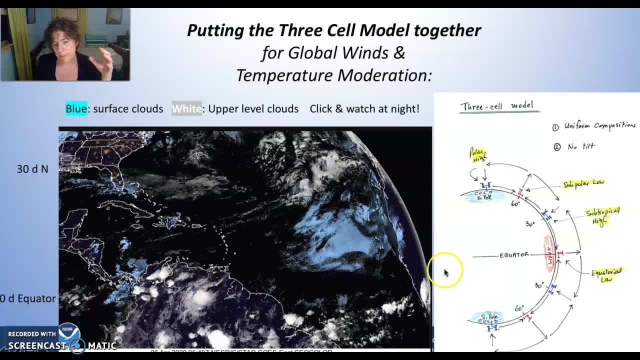 movements, movements. and you have here the equator, and you have here the equator, and you have here the equator. right along here. this is central america, right along here. this is central america, right along here. this is central america. this is the coast of africa. this is the coast of africa. 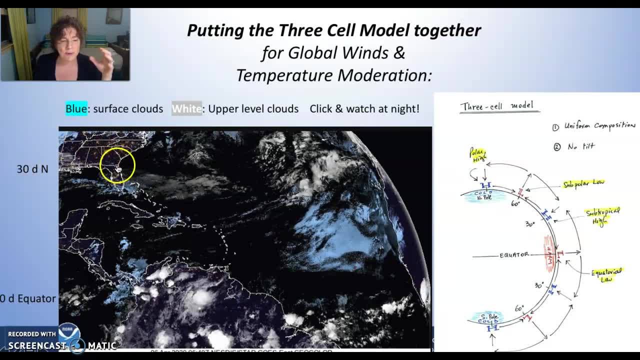 this is the coast of africa. you have here the 30 degree parallel, you have here the 30 degree parallel, you have here the 30 degree parallel. jacksonville, florida, jacksonville, florida, jacksonville, florida. tropica of cancer. we're talking about tropica of cancer. we're talking about 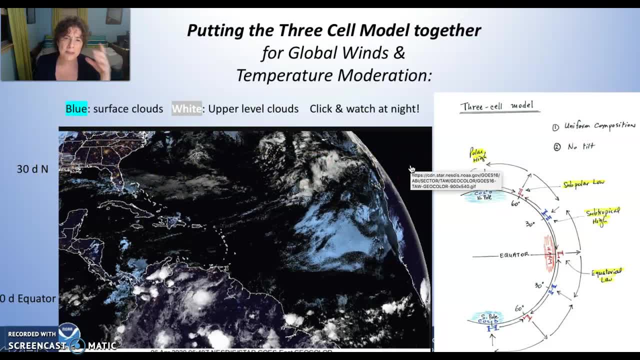 tropica of cancer we're talking about here, here, here, and so we have an area where we would, and so we have an area where we would, and so we have an area where we would expect to see surface trade winds, expect to see surface trade winds, expect to see surface trade winds coming from the northeast to the. 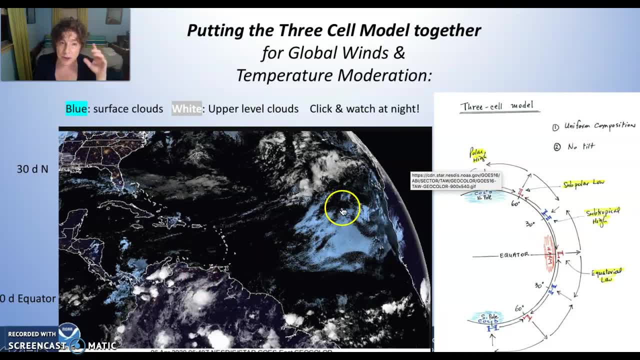 coming from the northeast to the, coming from the northeast to the southwest, southwest, southwest- and look what i see. i see surface blue and look what i see. i see surface blue and look what i see. i see surface blue: clouds, clouds, clouds in a direction that is coming from. 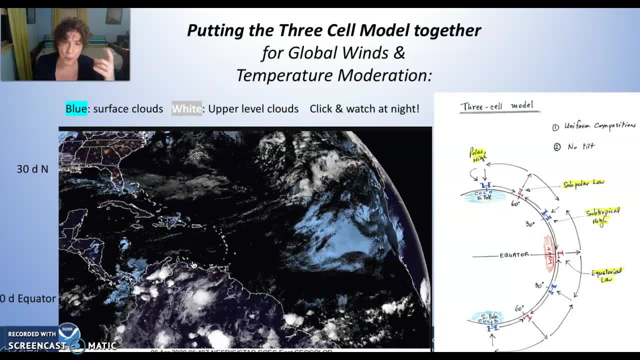 in a direction that is coming from, in a direction that is coming from the northeast to the southwest. those are the northeast to the southwest, those are the northeast to the southwest. those are northeasterly trade winds, northeasterly trade winds, northeasterly trade winds, right on the surface and right above it. 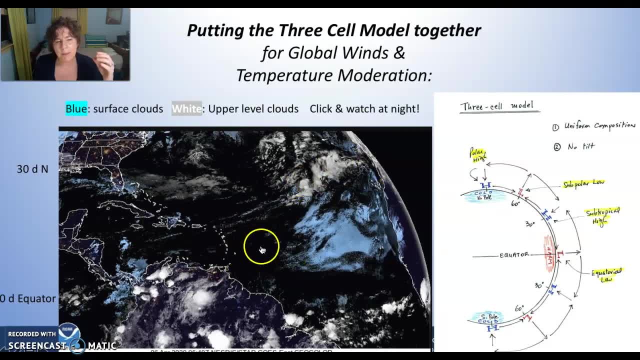 right on the surface and right above it, right on the surface and right above it, i start to see the higher clouds. i start to see the higher clouds. i start to see the higher clouds that are moving in a prevailing westerly, that are moving in a prevailing westerly. 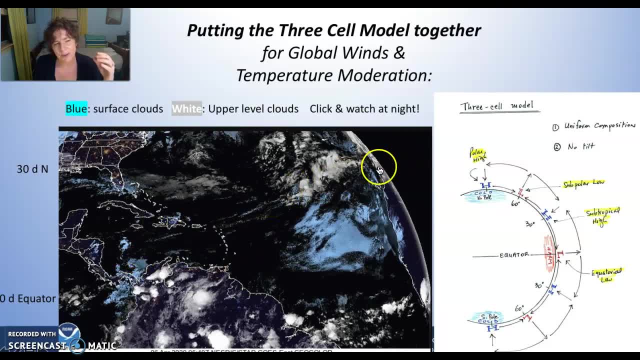 that are moving in a prevailing westerly fashion. fashion, fashion, those higher clouds, right there. they're those higher clouds, right there. they're those higher clouds, right there. they're beautiful, beautiful, beautiful. right, you see more prevailing westerlies. right, you see more prevailing westerlies. 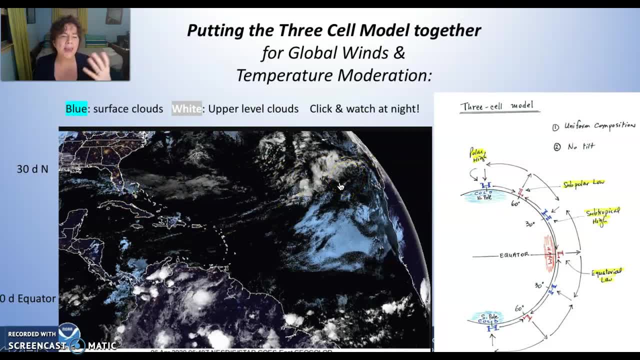 right, you see more prevailing westerlies up here, up here, up here, higher clouds. so here's a way that you higher clouds. so here's a way that you higher clouds. so here's a way that you can really see, can really see, can really see that this model starts to come into um. 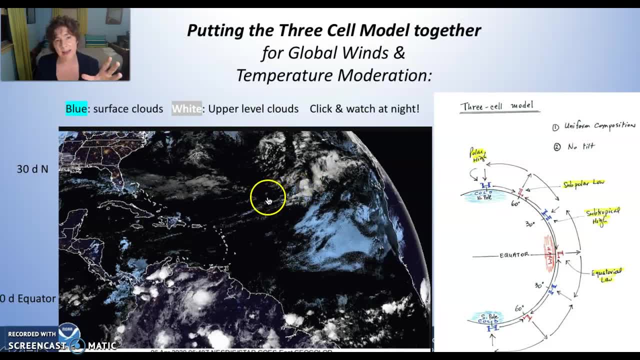 that this model starts to come into um, that this model starts to come into um effect. you can always look at the ghost effect. you can always look at the ghost effect. you can always look at the ghost satellite at night, satellite at night, satellite at night and look at the movement of air in. and look at the movement of air in and look at the movement of air in the hadley cell from the equator to 30. the hadley cell from the equator to 30. the hadley cell from the equator to 30 degrees degrees. 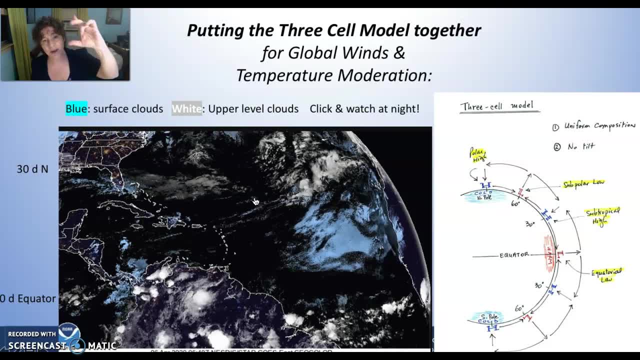 degrees. look at the movement of air in the. look at the movement of air in. the. look at the movement of air in the polar cell: 60 degrees. polar cell: 60 degrees. polar cell: 60 degrees to the north pole. have a look at it, to the north pole. have a look at it. 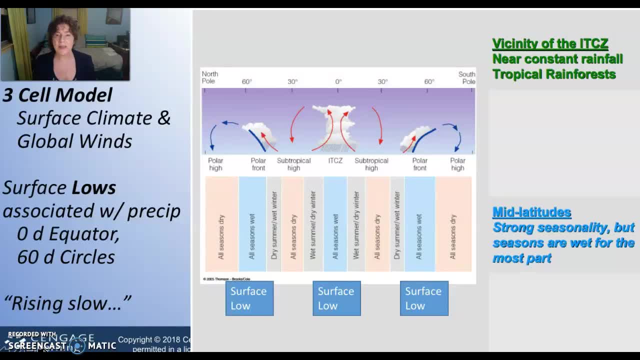 to the north pole. have a look at it. it's really wonderful to see, it's really wonderful to see, it's really wonderful to see, and i think that there's one more, i and i think that there's one more, i and i think that there's one more. i wanted you to wrap this up. 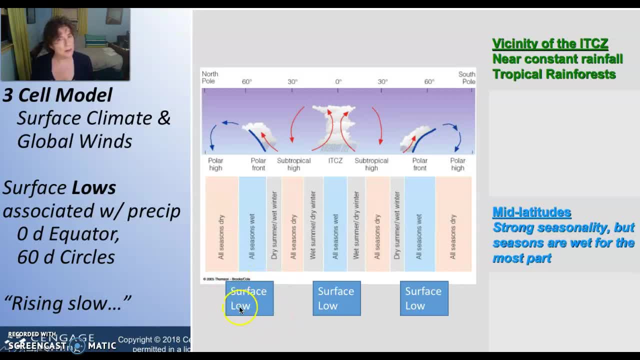 wanted you to wrap this up. wanted you to wrap this up by knowing that surface lows, by knowing that surface lows, by knowing that surface lows which are associated with the equator, which are associated with the equator, which are associated with the equator, and with 60 degrees. and with 60 degrees, and with 60 degrees: 60 degrees north, 60 degrees south, around 60 degrees north, 60 degrees south, around 60 degrees north, 60 degrees south, around the equator, the equator, the equator. those are associated with convection.